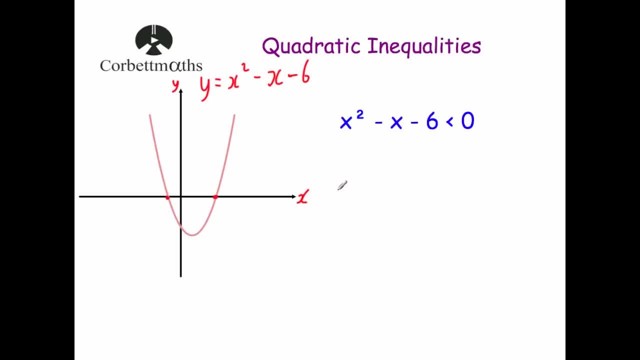 It crosses the x-axis. What we're going to do is we're going to get the graph, which is: y equals x squared minus x minus six. Now you want to find when it's equal to zero. so we're going to write: zero equals x squared minus x minus six. We'll factorize and solve it, So zero equals factorizing. 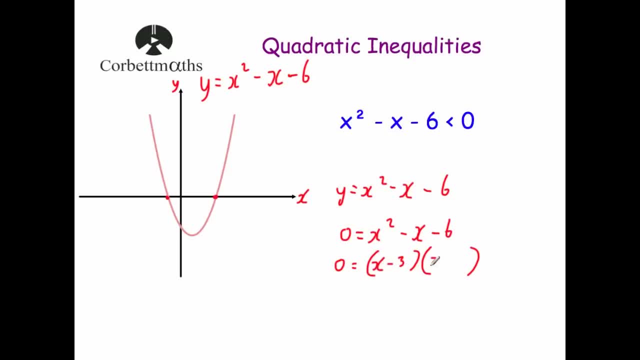 gives you x minus three, x plus two. Let's just check that: x squared plus two, x minus three, x is minus x, and minus three times two would be minus six. So that means our solution is x squared minus x minus six. So we're going to find out what our solutions would be. 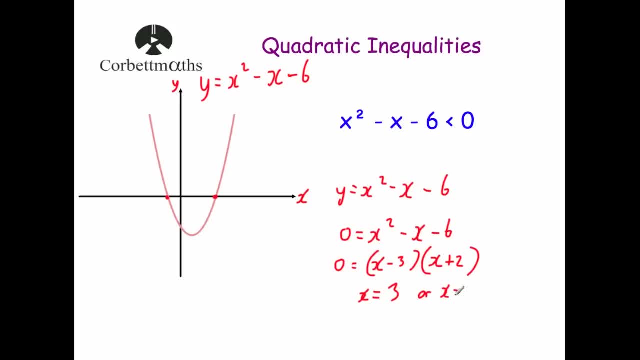 So our solutions here will be x equals three or x equals minus two. So that means that this point here is minus two and this point here is three. Okay, I'm just going to get rid of this for the moment, and what we're going to do is we're just going to explore what happens. Okay, so if I was, 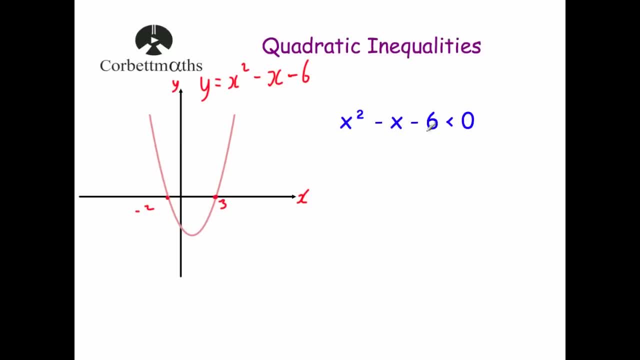 to substitute some values into this expression. this x squared minus x minus six. Okay so x squared minus x minus six, and let's see what we get. whenever I don't know x is equal to three, We'll know x is equal to three, We get x squared minus x minus six. 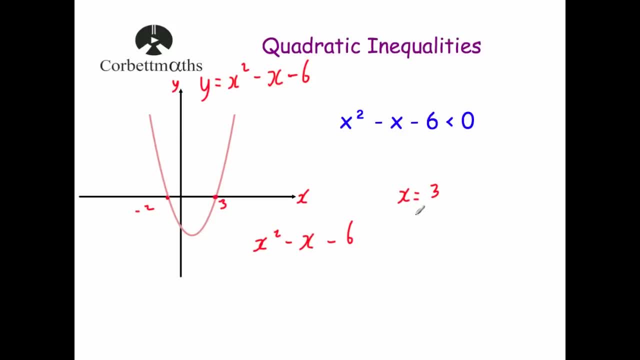 x squared, which is nine minus three, which is six minus six, which is zero. So the answer is zero and that's why it's there. If we go into, just say for instance this point here: whenever x is equal to two, x equals two, you get two squared, which is four minus two, which is two minus three, which is minus. 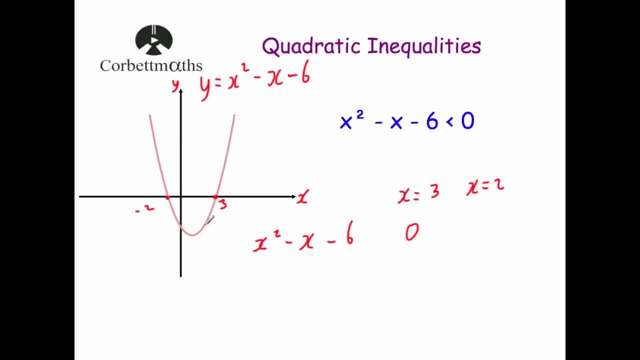 six, which is equal to minus four. So obviously you can see it's below the x axis because it's negative. If I was to try one zero minus one, I would get all negative values for that, or even for decimal numbers like minus 1.5.. 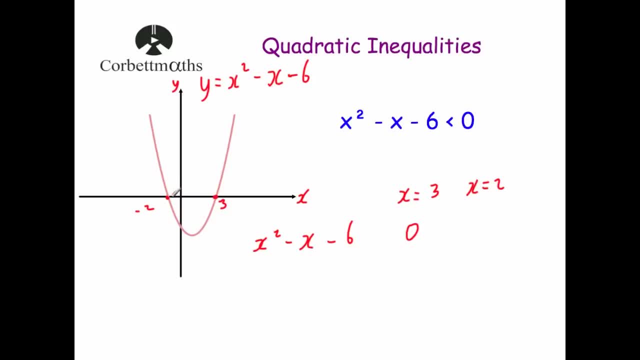 Minus 1.9, even minus 1.99 and so on. Okay, and again, minus two would give me the answer of zero. Okay, so what that means is, if I want to solve this inequality and this inequality of x, squared minus x minus six is less than zero. that means that any value here between minus two and three. 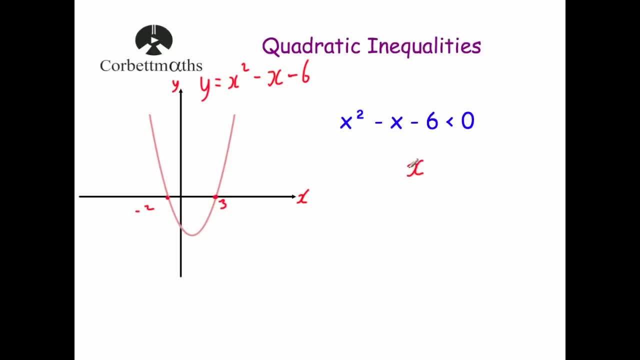 would give me a negative. So that means that x? my answer would be: x is going to be less than three, but it's going to be bigger than minus two, because that means that any value of x between minus two and three would work. It would give me a negative value. Okay, it obviously can't be minus. 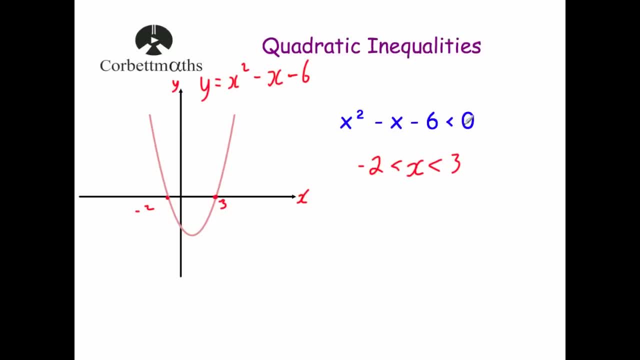 two or three, because they would be equal to zero, and this isn't less than or equal to zero, it's just less than zero. On that note, if I was asked to solve x squared minus x minus six is less than or equal to zero. my answer would be: because obviously this point here was three and this: 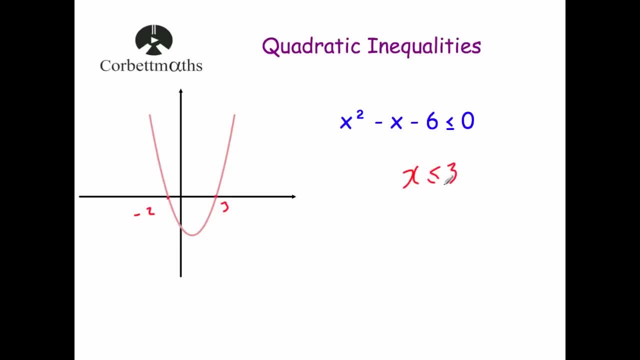 point here was minus two, the solution would be: x is less than or equal to three, but bigger than or equal to minus two, and that means that any value for x between minus two and three would be less than or equal to zero. Okay, let's have a look at the same inequality now, whenever it's. 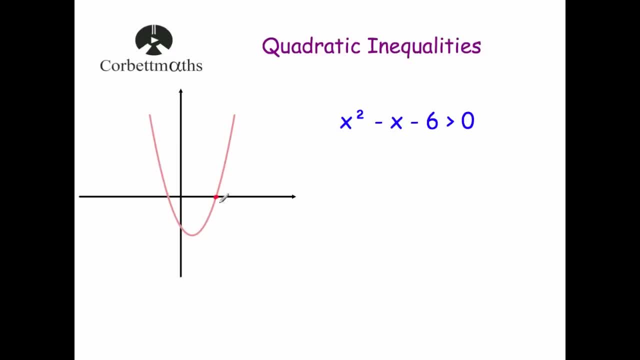 equal, bigger than zero. So again, we know this point here on the x-axis was three and this point here on the x-axis was minus two. Now we want to find which values give me a positive value. So positive values are whenever the graph of the function or the graph of the quadratic is above. 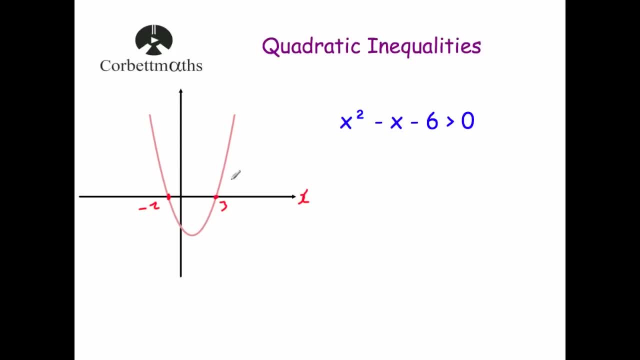 the x-axis. Okay, now we see we've got two distinct regions here. we've got to the right of three and to the left of minus two. Okay, so we've got two distinct regions here. we've got to the right of four. So let's just try putting in a value. let's just say x is equal to four. Okay, so if x is equal, 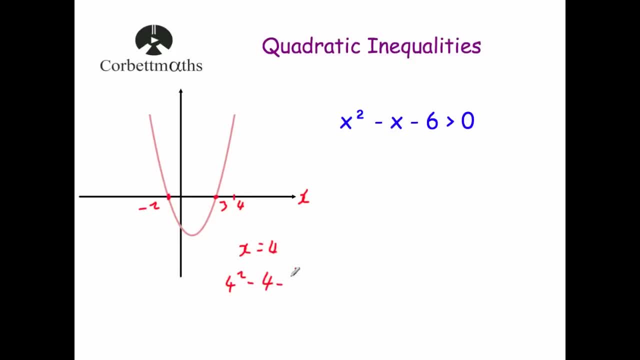 to four, that would be four squared minus four minus six. that'll be sixteen minus four minus six, and that would be twelve minus six that'll be. that's going to equal a value of six. As you can see, that's positive. if I was to try 3.5, it'd be positive. 3.1 positive, actually, any value bigger. 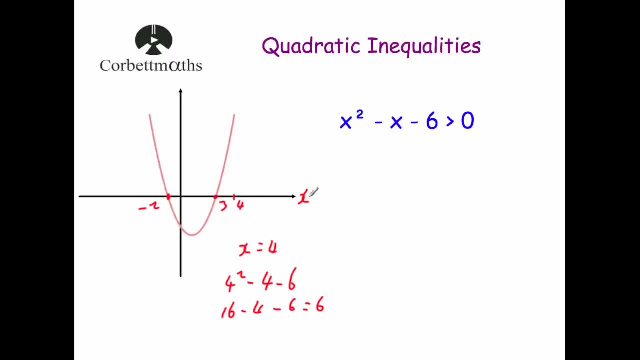 than three would be positive, and that would go on forever. for instance, a hundred, a million and so on. because a quadratic graph has a u-shape, it will just carry on going up. So that means that one part of my solution will be any value of x which is bigger than three, but also 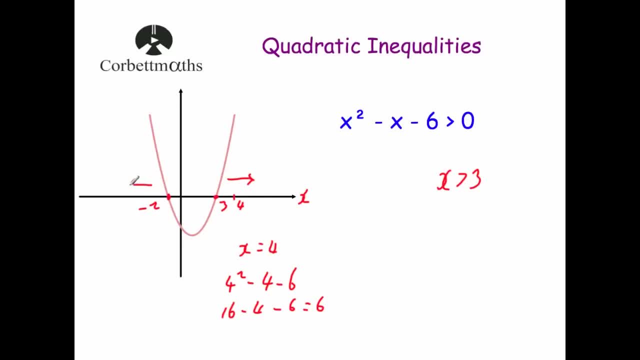 we've got this section here, Okay. we've got this bit to the left of minus two, Okay. so it means, for instance, if I was to try a value smaller than minus two, perhaps minus three, let's see what we get. So whenever x is equal to minus three, well, minus three squared negative times, negative is: 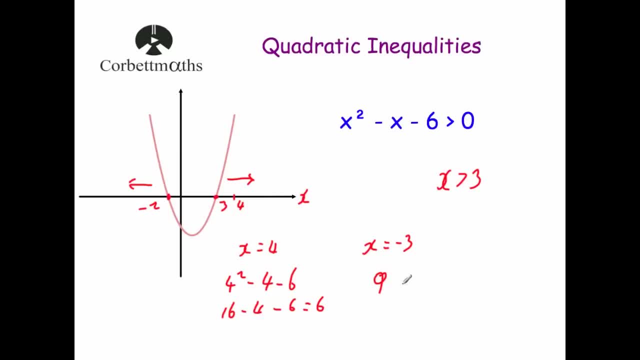 a positive, that's nine minus x. that's going to be minus minus three, which would be plus three, and then minus six. So it's going to give me twelve and then take away six would be equal to six. So again, if I was to try minus three, it gives me a positive, Minus four would be. 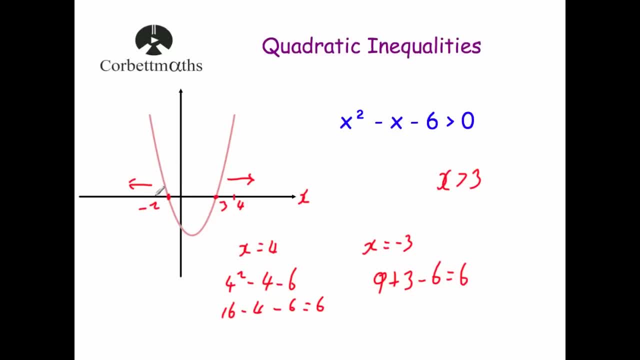 positive and carry on forever would be positive, Even minus, you know, minus 2.1, minus 2.01 and so on, Just any value that is less than minus two. Now we can't write that as one inequality. so what we do is we write our answer like this: We say that x is going to be smaller than minus two, or x is 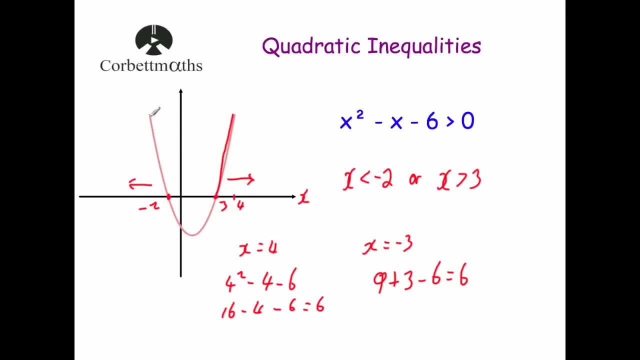 bigger than three because we've got two distinct regions. We've got this region and we've got this region. So we write it as two different answers. We say that x is going to be smaller than minus two, or x is less than minus two, or x is bigger than three, And likewise if it was bigger than equal. 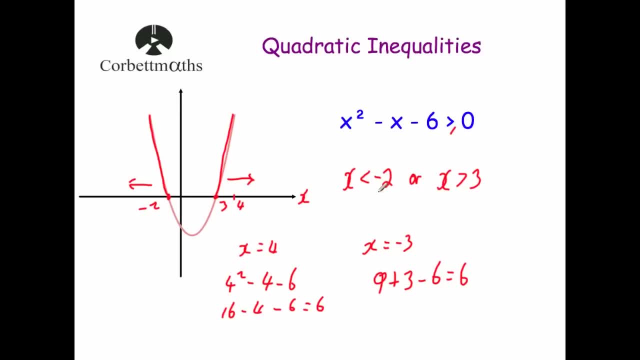 to zero. what we would do is we, if it was bigger than equal to zero, it'll be. obviously it means it can be zero as well. We know that the graph, or the, the quadratic, is equal to zero minus two and three. So we could put the little line there and the little line there and we could say that x is. 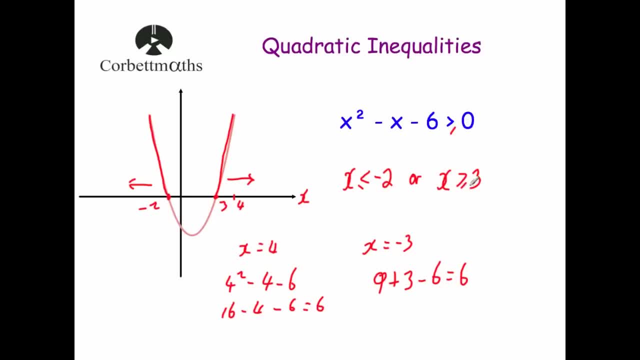 less than or equal to minus two, or x is bigger than or equal to three. Okay, let's have a look at some questions. So our first question we're going to try is this one here- To solve the inequality: x squared plus 2x minus 15 is less than zero. So, again, what I want to do is I: 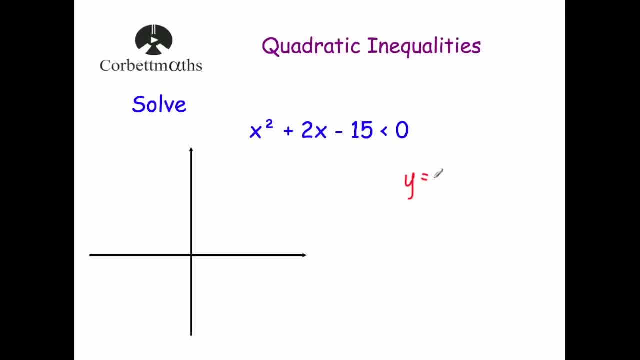 want to sketch the quadratic graph. So what I'm going to do is I'm going to let y equals x squared plus 2x minus 15, and I'm going to draw that graph. Let's let it equal zero to find the key values. 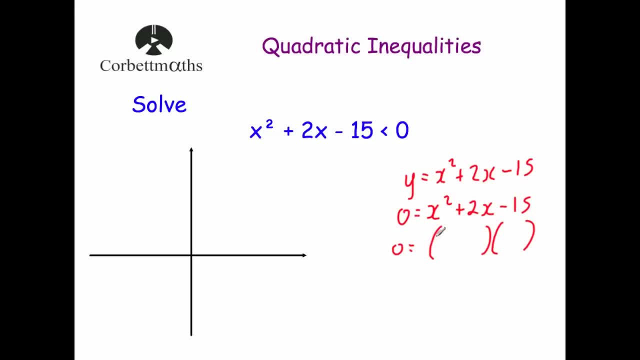 So let's again factorize and solve it. So factorizing x, x, and if it didn't factorize you'd use the quadratic formula. or if you're completing the square, So x, x, and it's going to be plus 5 and minus 3, and that means that the values for x will be x equals. 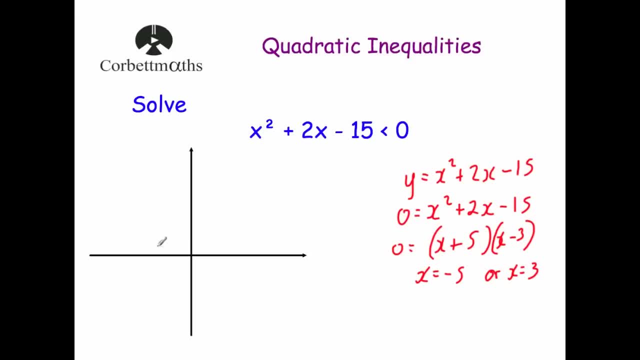 minus 5 or x equals 3.. So that means it's going to cross the x axis at minus 5 and it's going to cross again at 3.. Okay, so sketching the quadratic graph. it will come down through there and then come back up again and through there. Okay, please excuse my quadratic graph sketching. Okay, now we're. 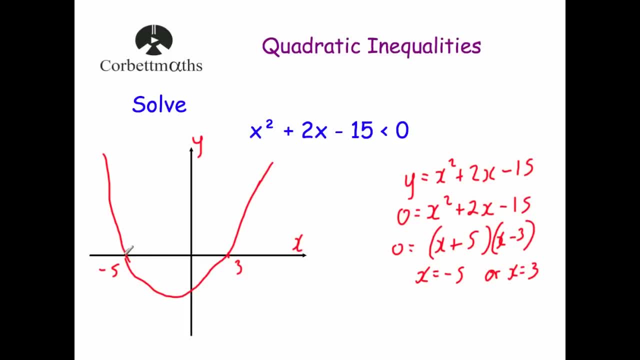 trying to find when this quadratic is less than zero. Okay, now you can see, it's less than zero between minus 5 and 3.. Okay, so that means, for instance, minus 4 would work, minus 2 would work, zero would work, two would work, one would work. Obviously it's less than zero. so 3 and minus 5. 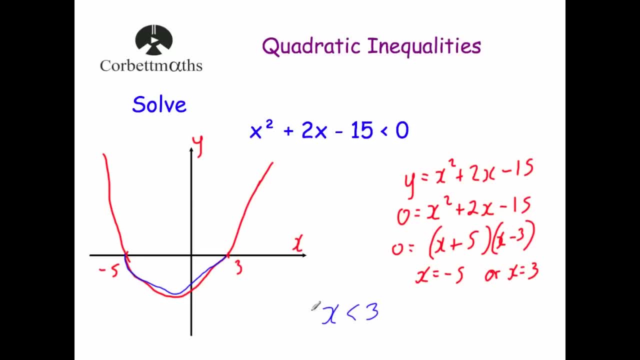 themselves won't work. That means that x is going to be any value that is less than 3, but it's bigger than minus 5, and that's it. That's that quadratic inequality solved. Next I solve x squared minus 9x plus 18 is bigger than zero. Okay, so again, let y equals x squared. 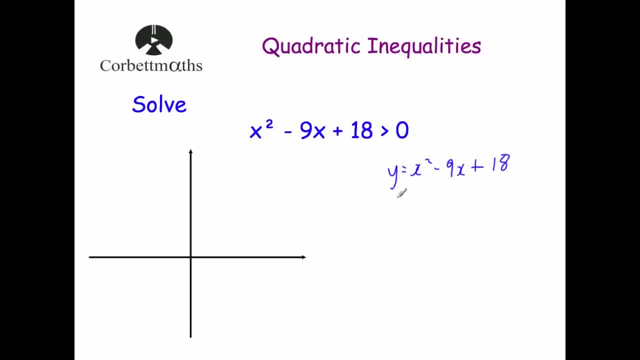 minus 9x plus 18 and we'll draw this graph. So that's going to be zero equals. to find where it crosses the x axis, We're going to let it equal zero. So x squared minus 9x plus 18 and we'll. 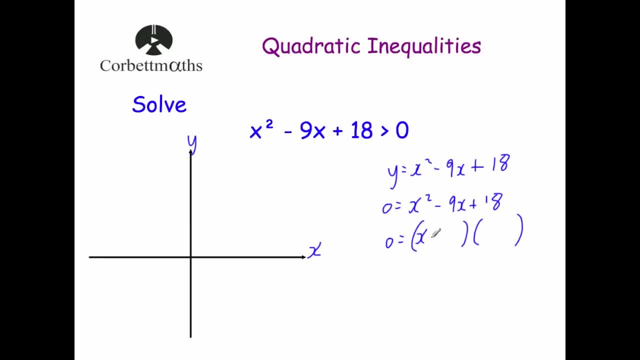 factorize it, It's going to be x minus 3 and x minus 6.. So that means x equals 3 or x equals 6.. So it means it's going to cross the x axis at 3 and 6.. And again, it's an x squared graph. so it's: 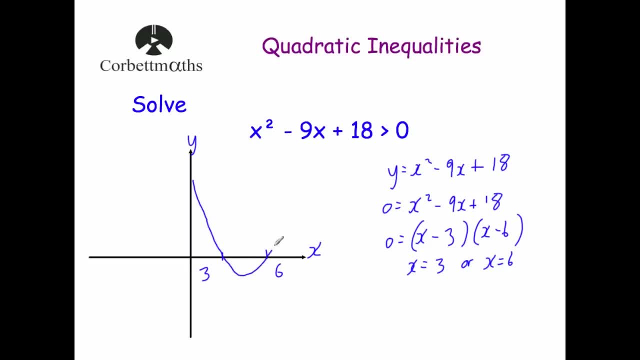 going to come down and then back up again, like so, If it was a minus x squared in the question, you could just bring it all to the other side. That's personally what I would do. I like just drawing the u-shaped quadratic. so it's bringing them all over to the other side, Or you could. 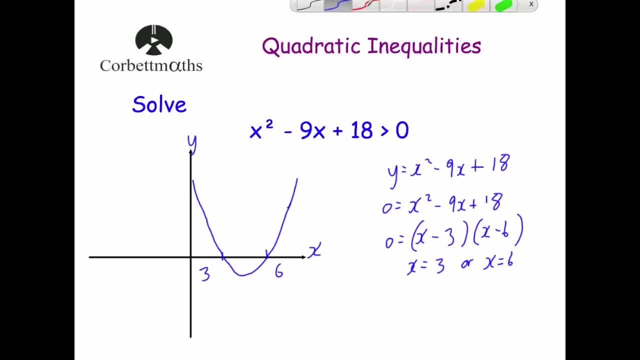 draw the quadratic, but remember it'd be an n-shape. Okay, so let's just draw this. We've drawn this quadratic. We want to find this time when it's bigger than zero. So bigger than zero is when the graph, or when the graph of the expression, is above the x axis. 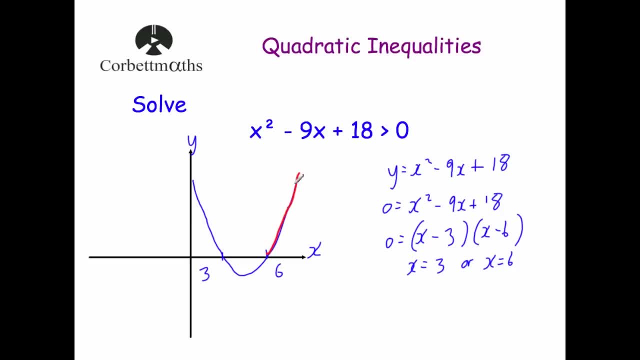 So, as you can see, it's above the x axis at this section and this section here. Okay again, excuse me drawing. So here we've got any value for x which is bigger than 6, because obviously 6 is zero. We want it whenever it's bigger than zero. So 7 would work, 8 would work, 9 would work and so. 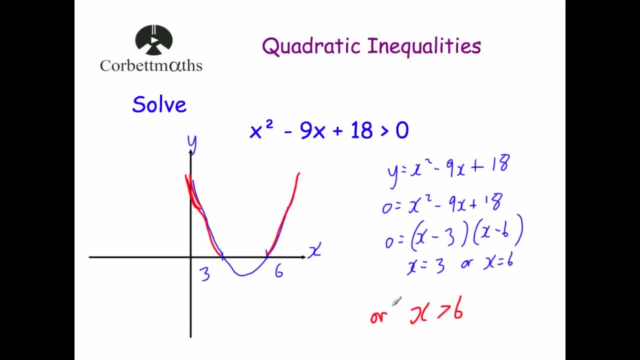 on. So we're going to say that x is going to be bigger than 6.. Or, obviously, any value less than 3 works as well. So 2, 1, 0 and so on. So x is less than 3.. Because it's two different regions. 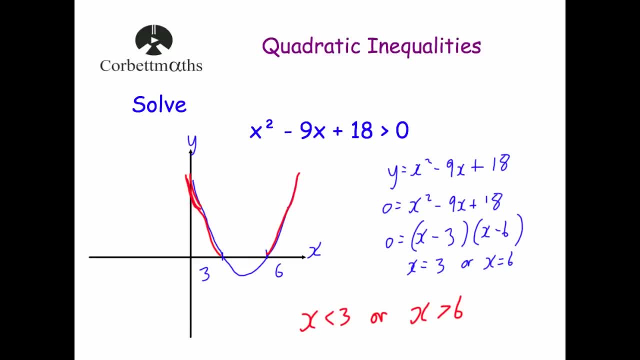 x is less than 3 or x is bigger than 6.. And the last question. It says: solve 4x squared minus 7x plus 20 is less than x plus 17.. Now the way I solve these ones, whenever it's not a zero, is I.